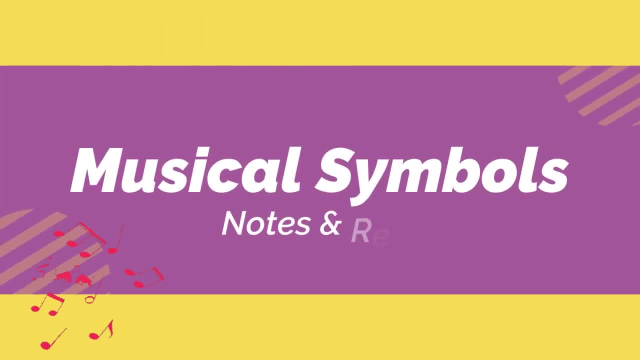 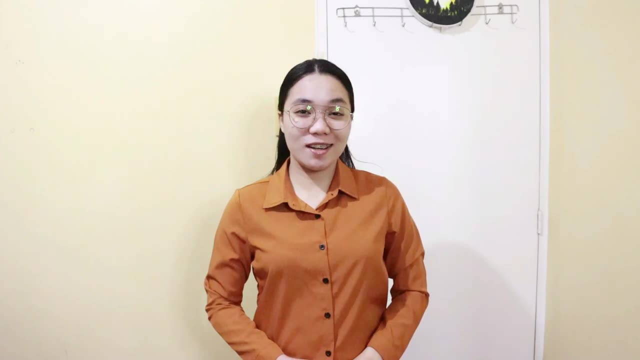 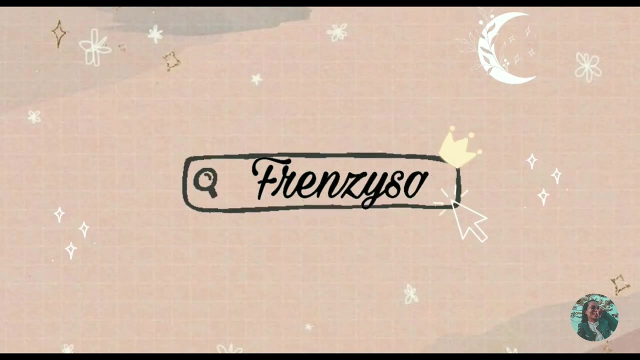 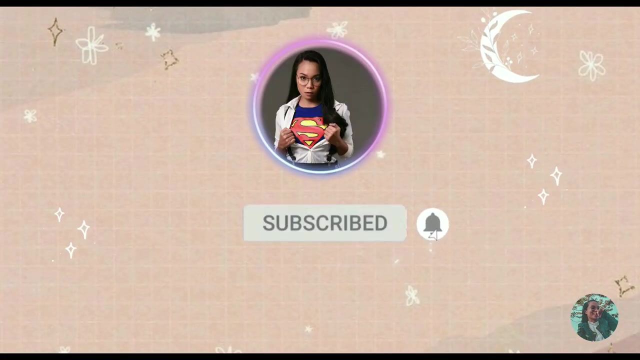 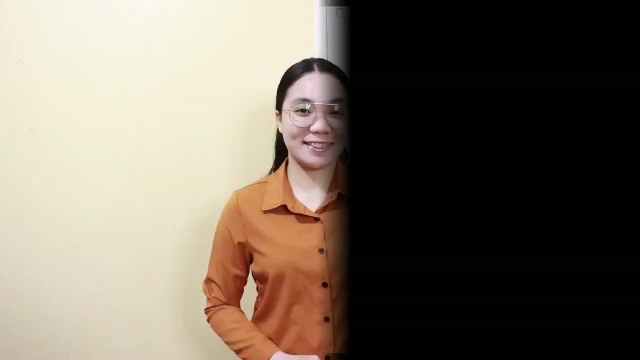 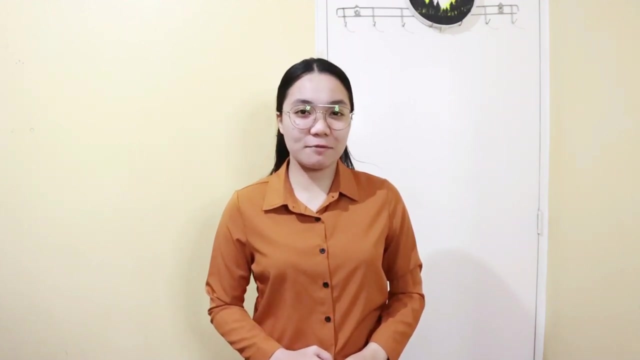 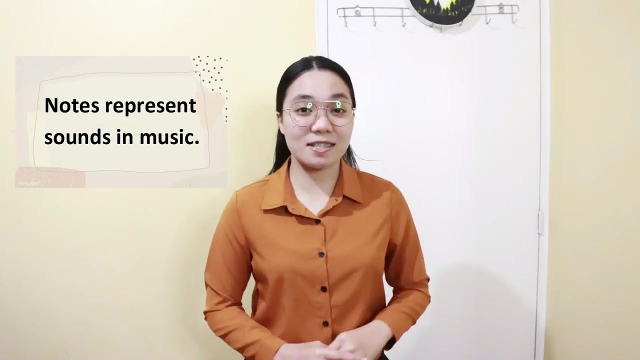 Good day everyone. Welcome back to my channel. This video will help you to learn and master the different kinds of notes, rest and their time values. Notes represent sounds in music, while the rest is the opposite of it, So the rest represent silence in music. 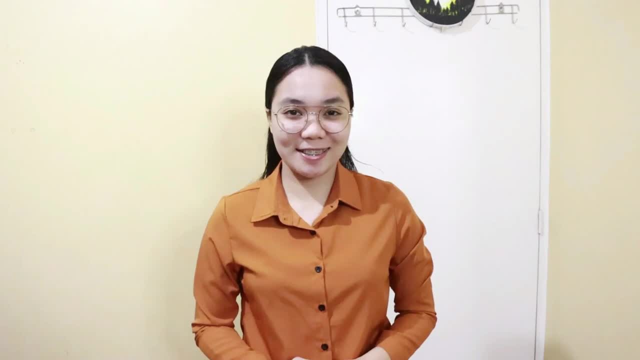 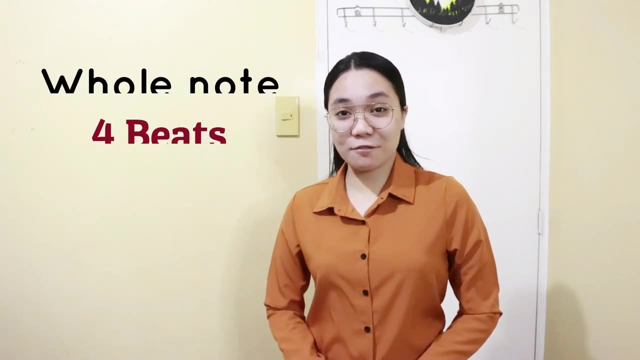 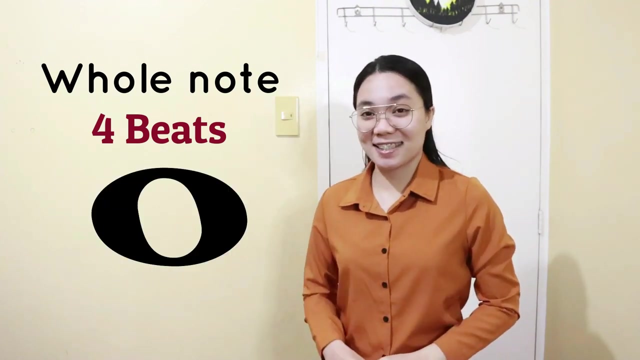 So let's begin with the different kinds of notes. The first kind of note we have is what we call silence Whole note. Whole note has a time value of 4 beats And it is the longest time value of all notes, And it looks like this: 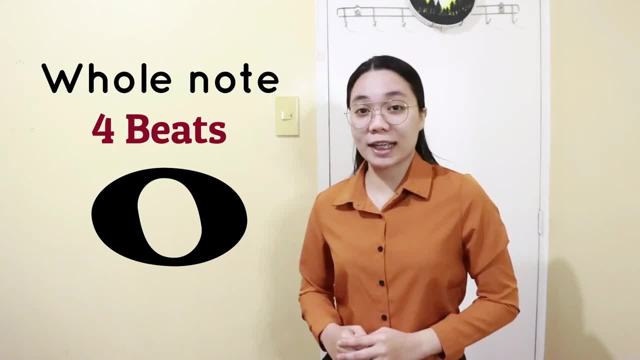 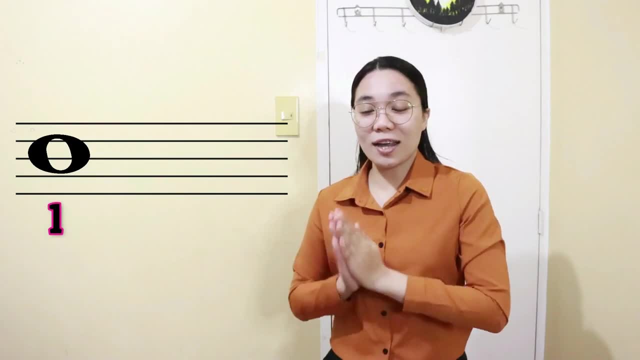 As what is said, whole note receive 4 beats or 4 counts, And it sounds like this: 1, 2, 3, 4.. 1, 2, 3, 4.. 1, 2, 3, 4.. 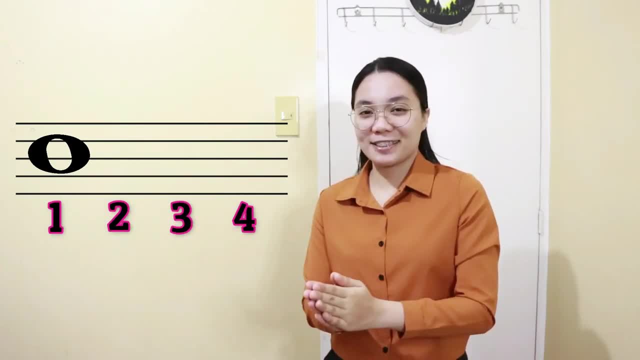 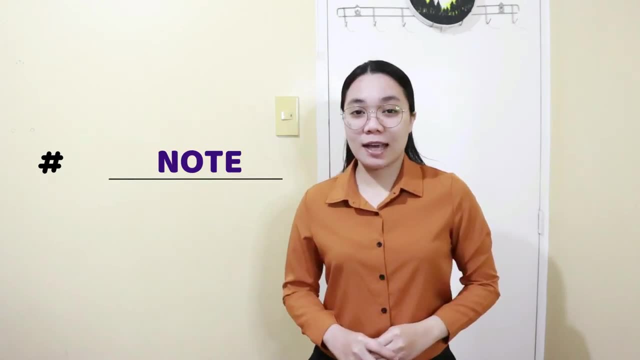 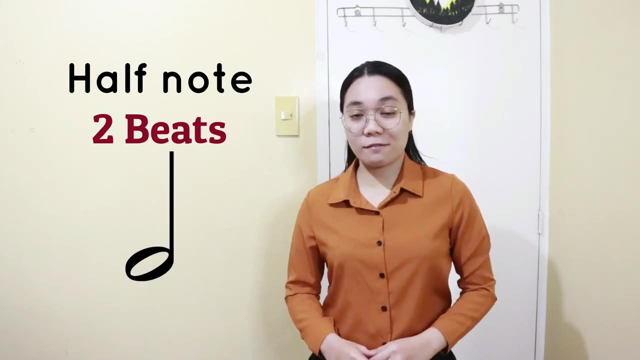 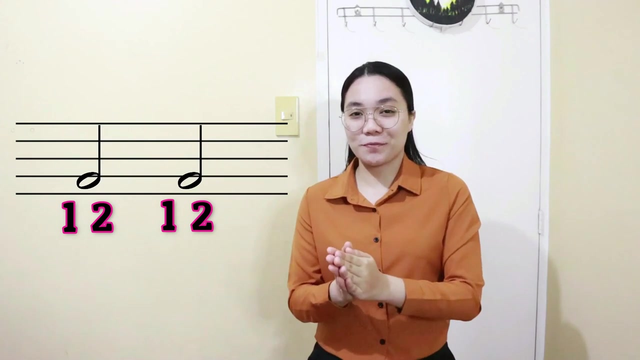 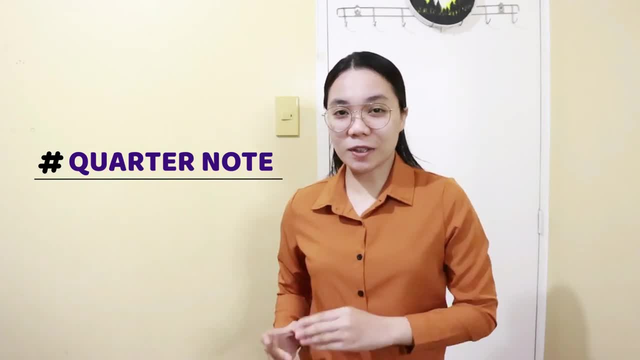 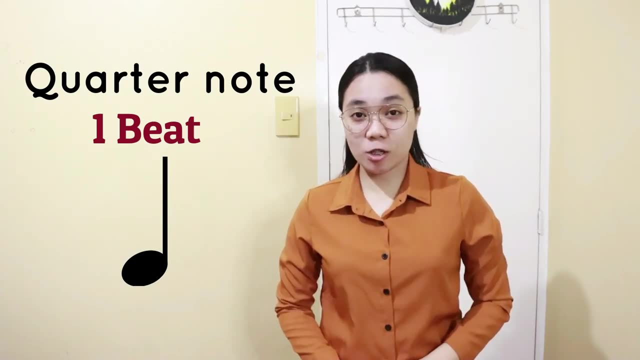 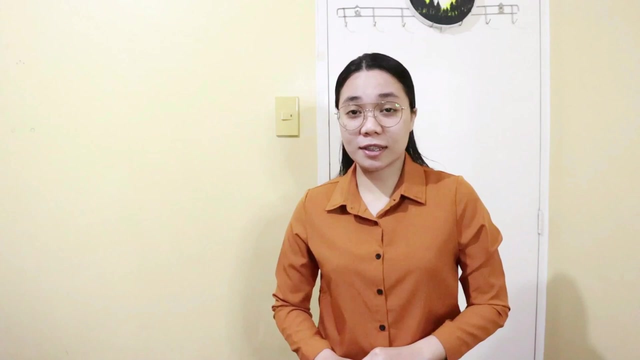 Next note is what we call quarter note. Quarter note receives 4 beats. Quarter note receives 1 beat And it looks like this: As you can see, the head of a quarter note is already shaded compared to half note, So let's go back to the time value of quarter note. 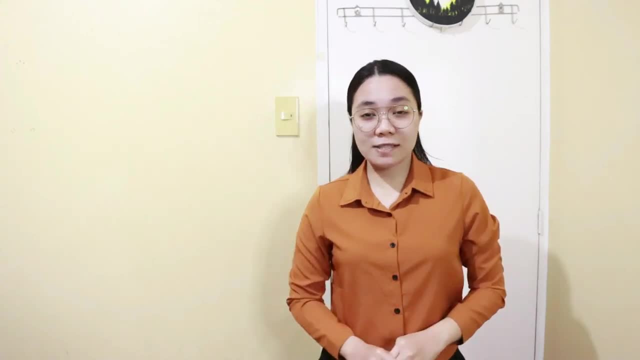 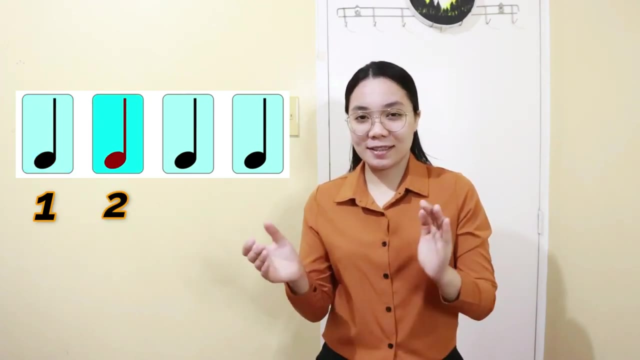 It receives 1 beat. For example, if we have 4 quarter note, it sounds like this: 1, 2,, 3, 4.. 1, 2, 3, 4.. 1, 2, 3, 4.. 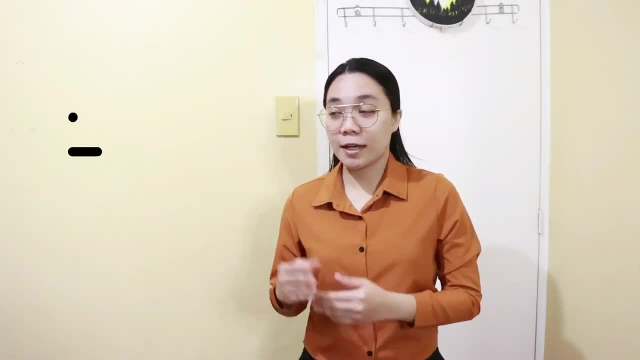 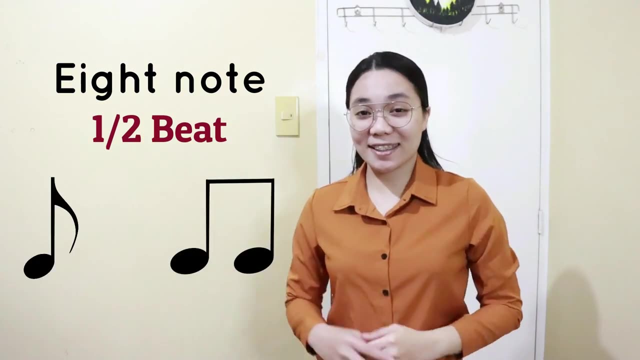 So let's proceed to the next kind of note, What we call eighth note. An eighth note has a time value of 1 half beat And it looks like this: As you can see, eighth note are rotated with an oval shaded head with stem and 1 flag or 1 hook. 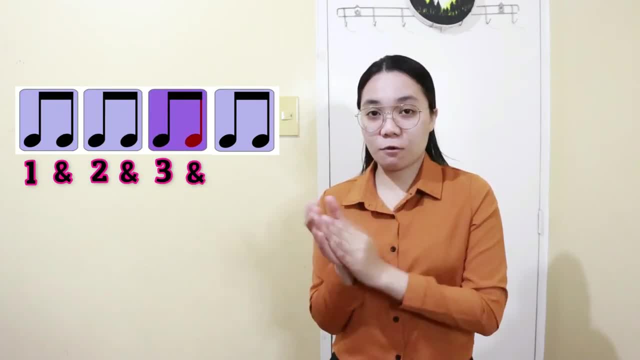 And it sounds like this: 1 and 2 and 3 and 4.. Again, 1 and 2 and 3 and 4.. 1 and 2 and 3 and 5 and 7 and 8 and 9 and 10.. 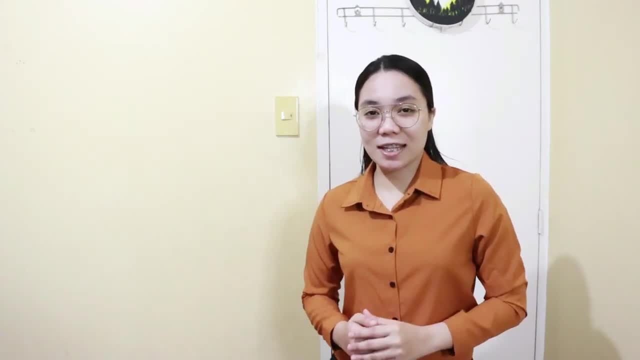 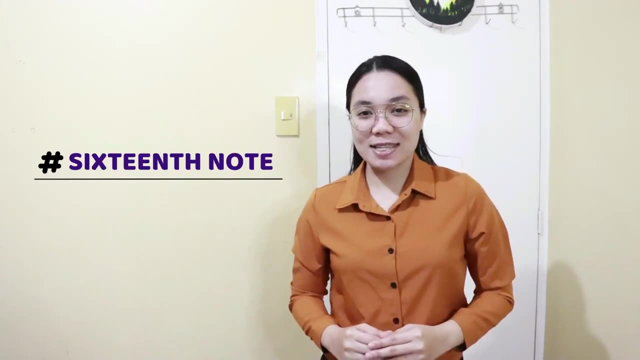 1 and 2 and 3 and 4.. went 3 and 4 red. So that is the beat of eighth note with one half beat, And our last note is what we call sixteenth note. Sixteenth note has a time value of one fourth beat and it looks like: 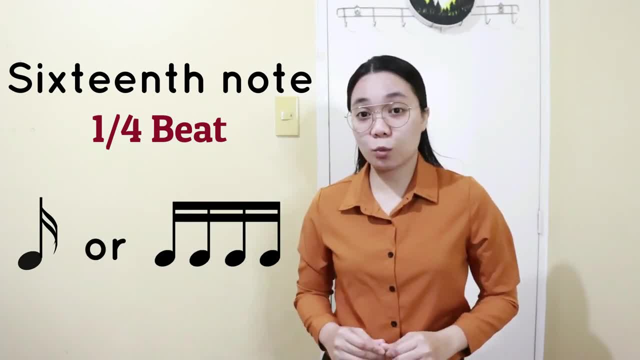 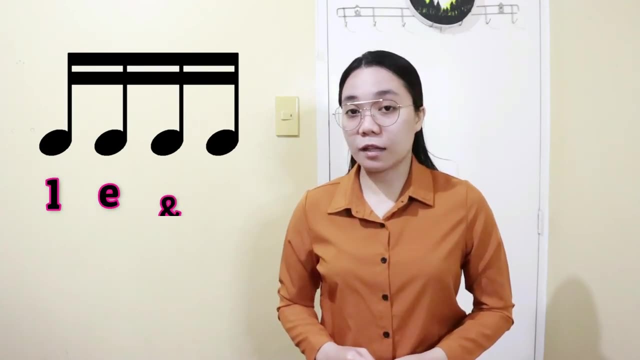 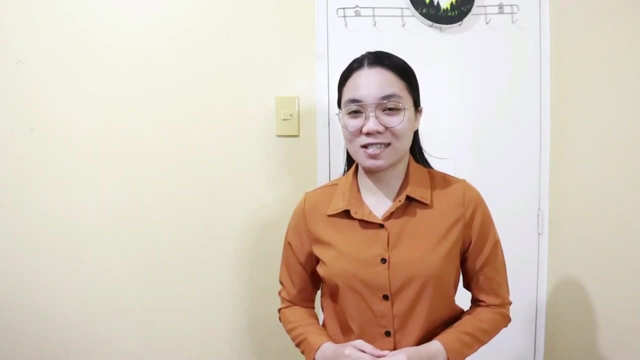 this. So sixteenth notes are also dated with an oval shaded head with stem and two flags or two hooks. For you to follow the right beat of this sixteenth note, you can use this pattern: One e and a, Again one e and a, And it sounds like this: One e and a, two e and a three. 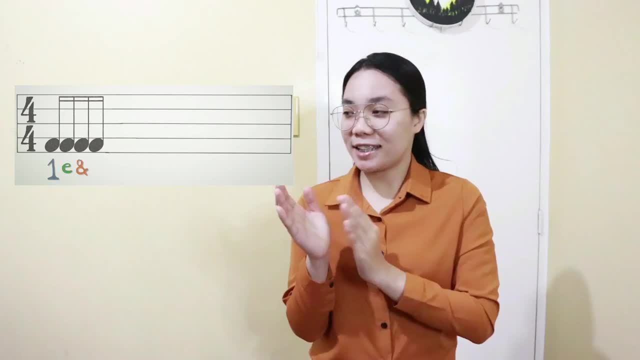 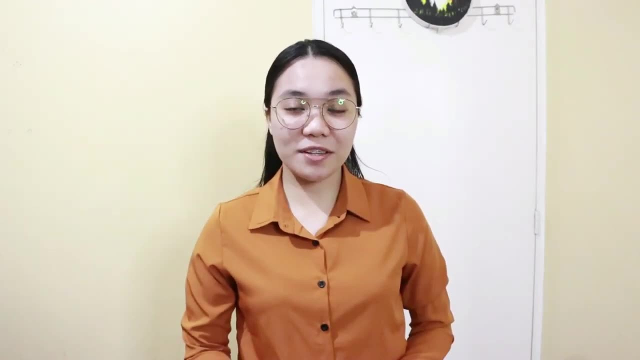 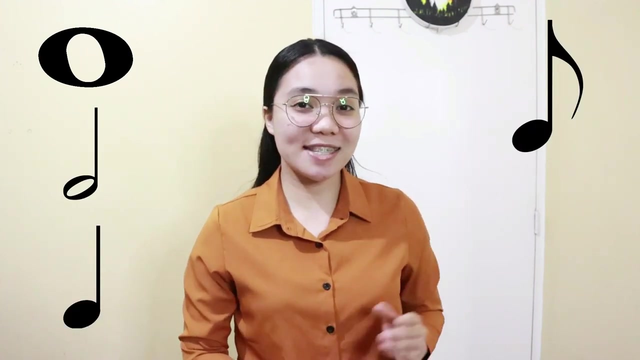 e and a four e and a. Again one e and a two e and a three e and a four e and a. Okay, so our different kinds of notes are whole note, half note, quarter note, eight note and sixteenth note. 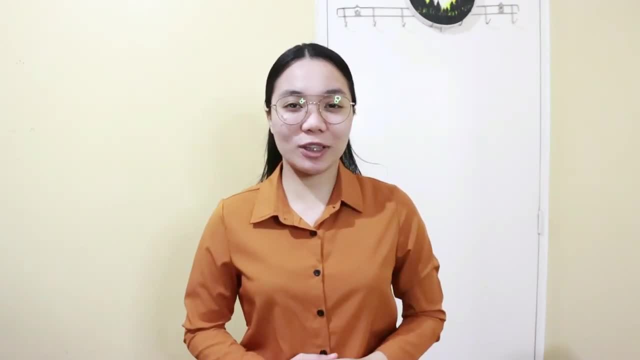 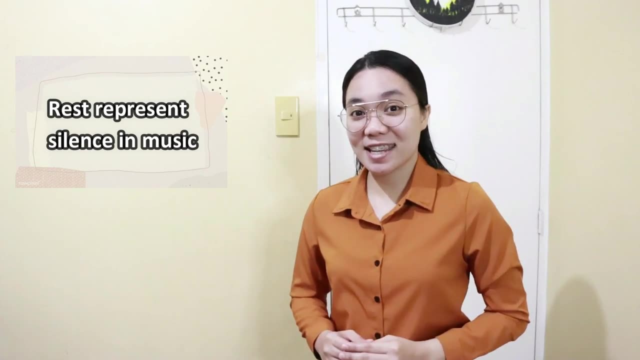 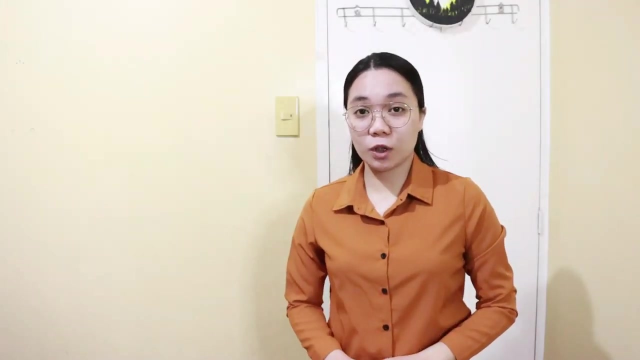 So now let's move on with the different kinds of rests. When we say rest, it represents silence in music, Shh. So the first kind of rest is what we call Whole rest. As you notice, the names are types of wrestling and Fire avant-garde, which also holds. 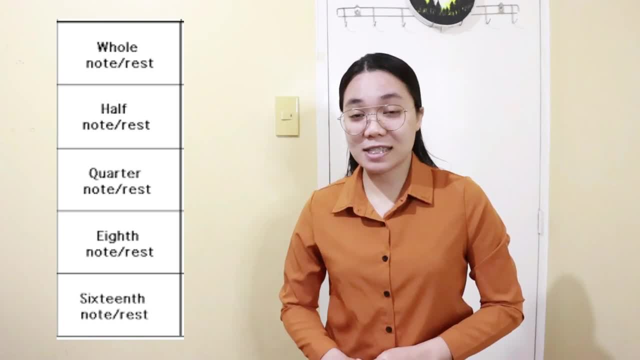 we call the whole dance part out And just walk around. that didn't feel like taking your. So the first kind of rest is what we call a rest function, and we also fall in love with what you see. notes are almost same. the only difference is that you just replace the. 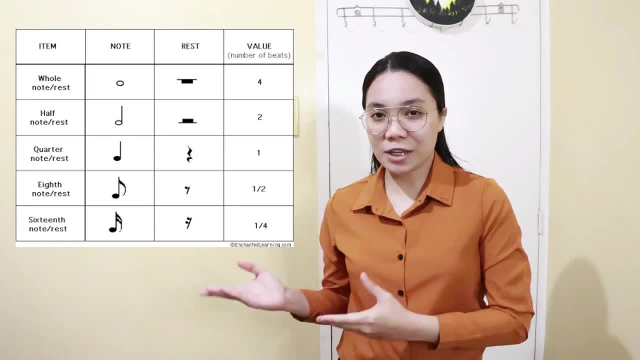 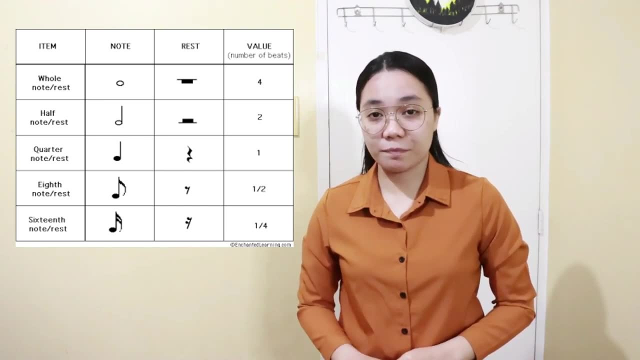 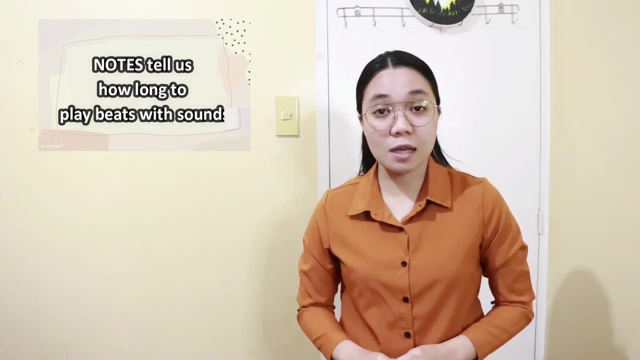 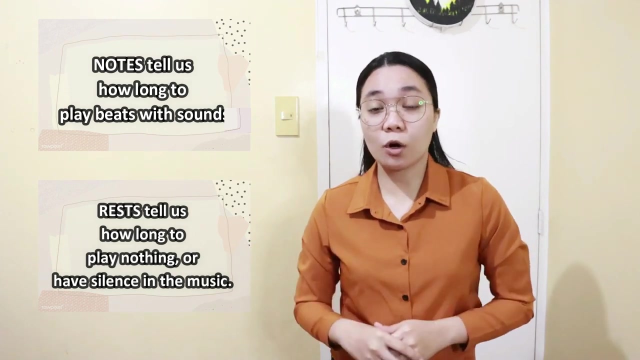 word note to rest. so here is the example table. as you can see, the names and the time values are the same. but always remember notes tell us how long to play beats with sounds, while the rest tell us how long to play nothing or have silence in music. I don't think you will be confused between the notes and rest. 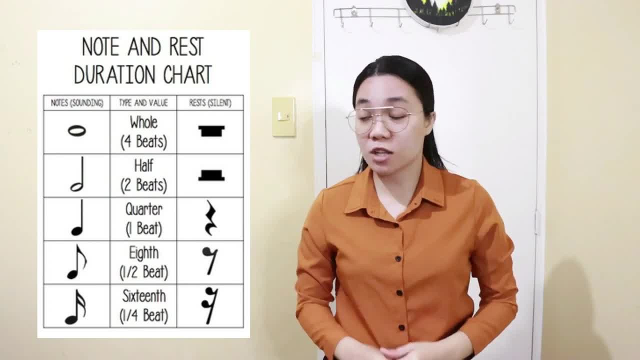 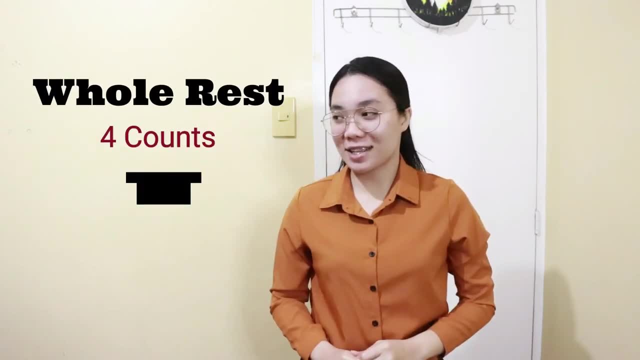 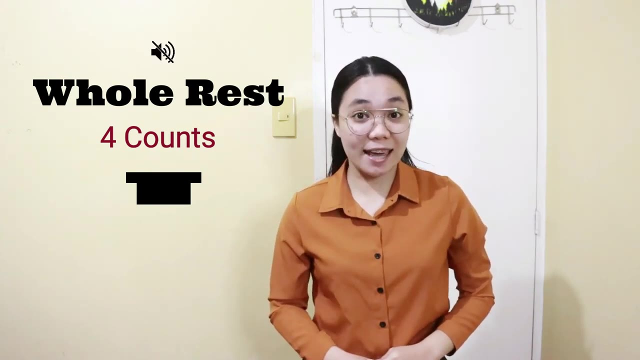 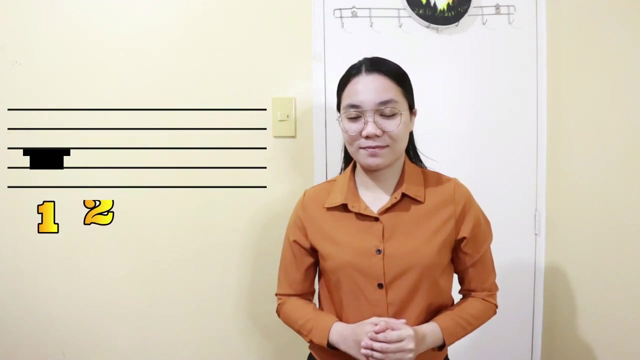 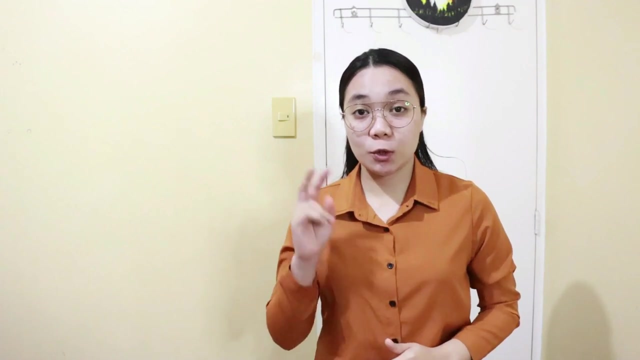 because the symbols are different, as you can see here in the table. so let's discuss it one by one. let's go back with the whole rest. it receives four beats like cool note, four beats in silence. so here is the example. okay, next is half rest and it receives two beats and silence. for example, 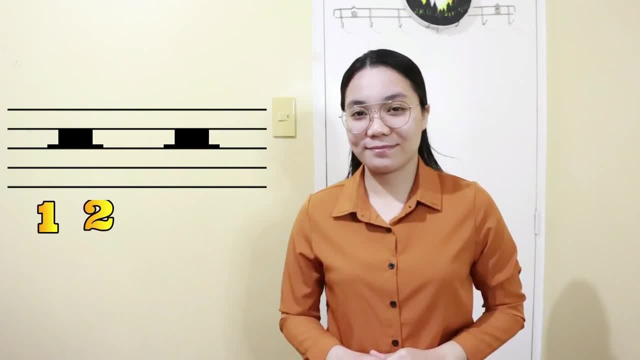 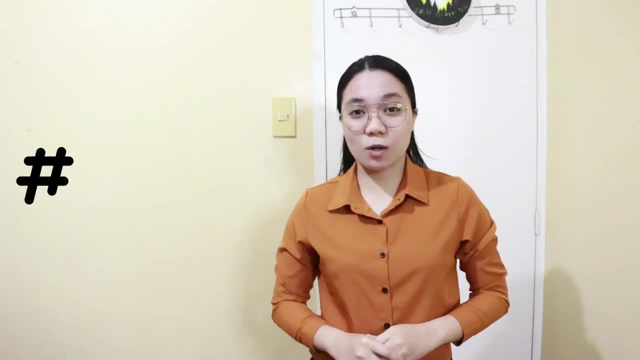 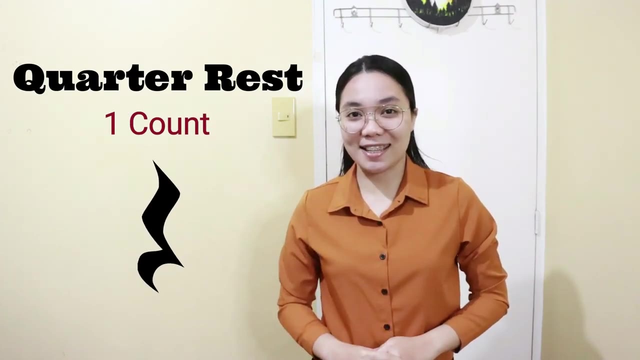 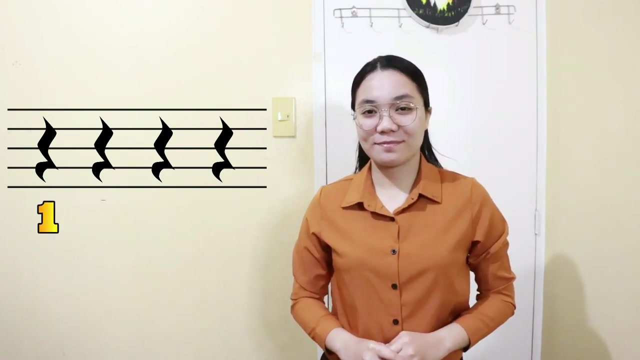 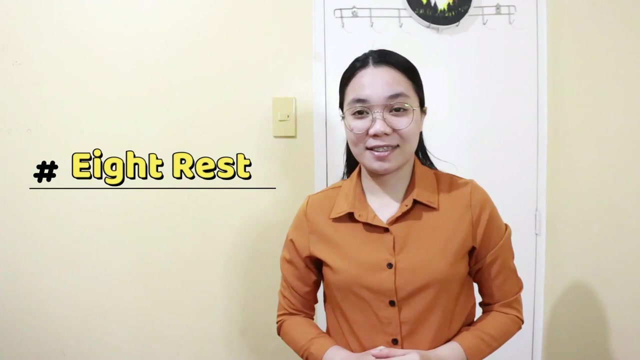 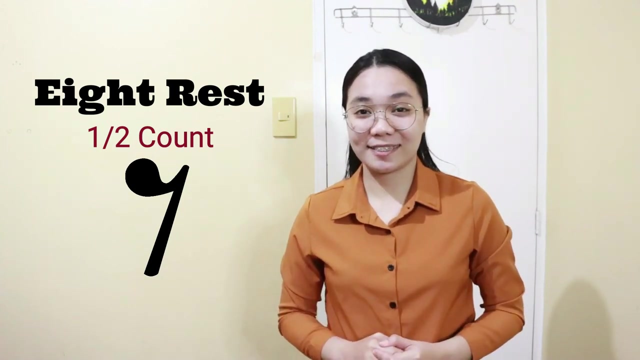 next is the quarter rest, and this is the symbol of quarter rest: it receives one bit in silence. so here is the example: you, you, you, you. Next kind of rest is what we call 8 rests. It has a time value of 1 half-bit and it looks like this: 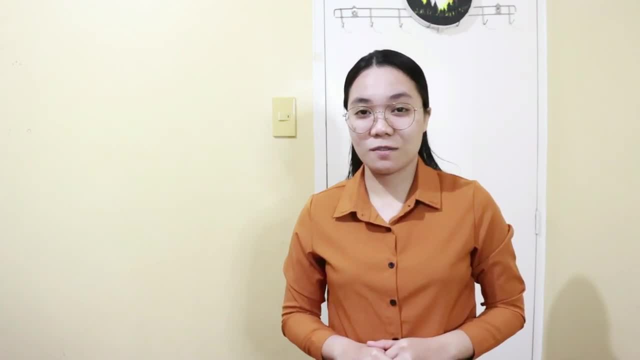 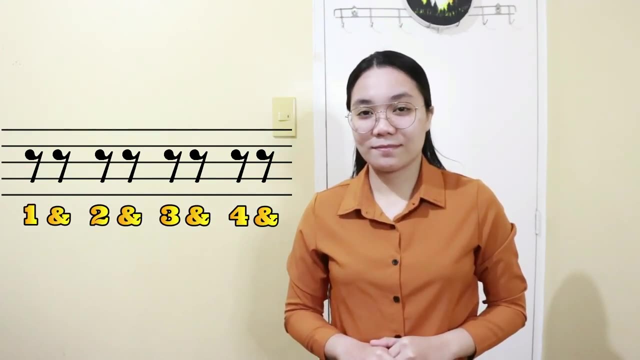 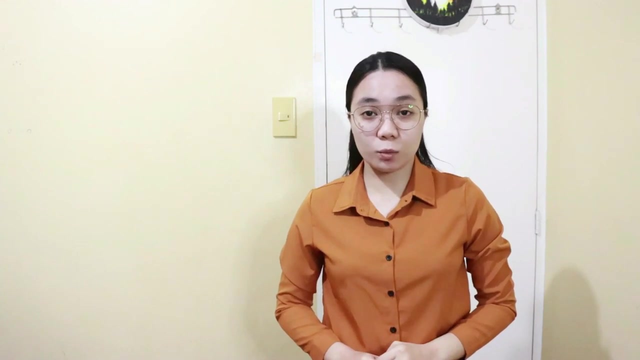 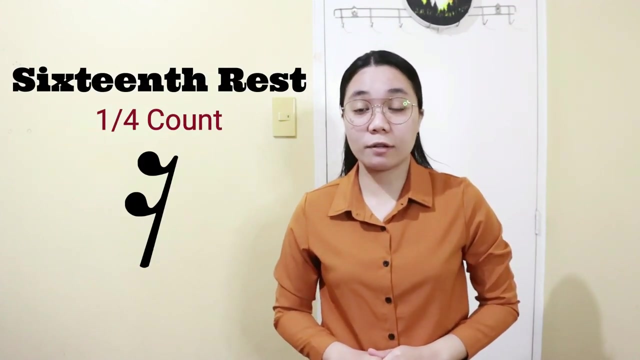 And this is the example of 8 rests. And our last kind of rest is what we call 16th rest. Just like a 16th note, it has a time value of 1 fourth-bit, Again in 16th note. you have to follow this pattern. 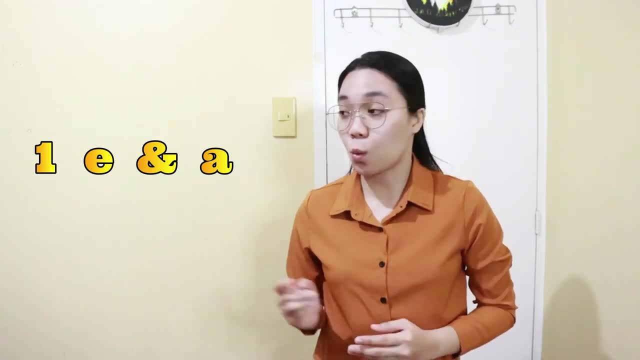 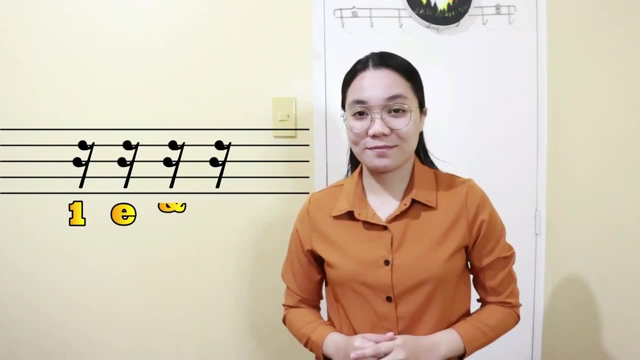 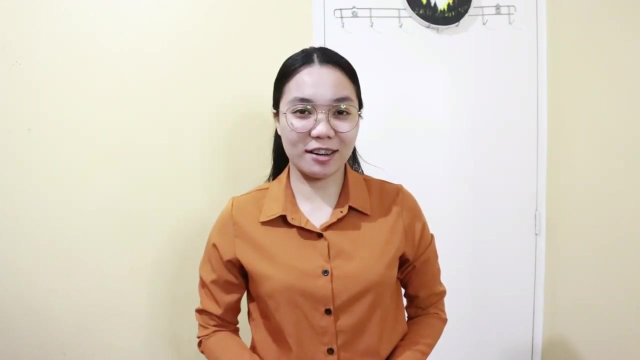 For you to be able to follow the right beat. so 1, E and AH. So here is the example. So our different kinds of rests are full rest, half rest, quarter rest, 8th rest and 16th. 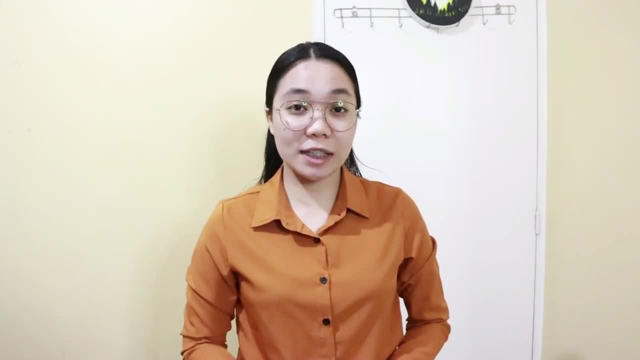 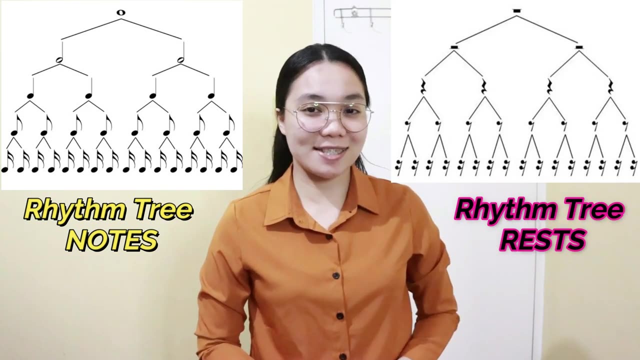 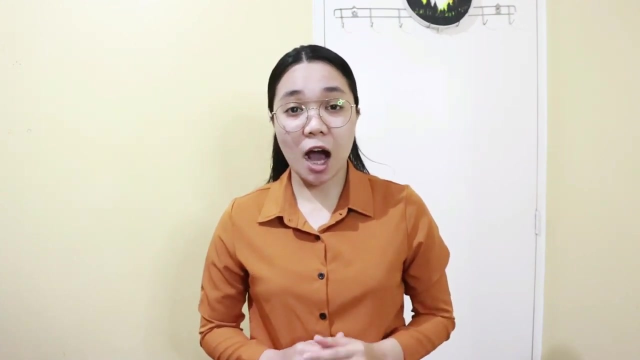 rest. There you have it Now. you already know the different kinds of notes and rests. So these are the rhythm tree notes and the rhythm tree of rests. Another information: when dots are seen beside a note or rest after its time value to increase. 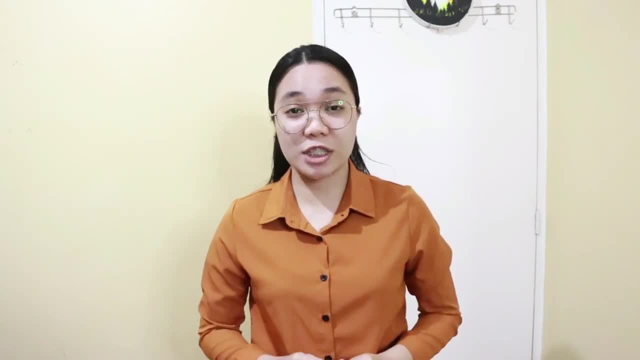 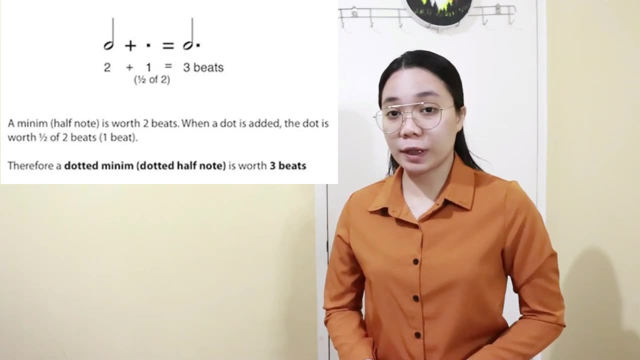 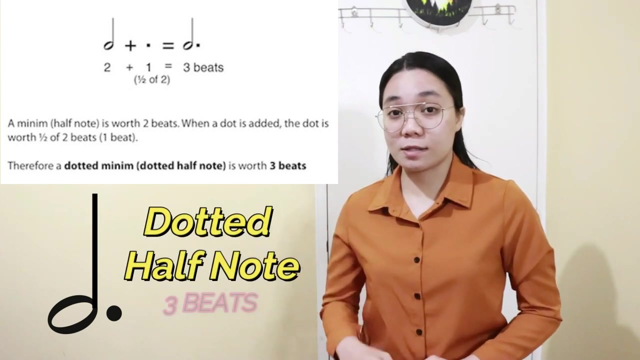 the original beat of a note or rest by half of the original values. Let's see this example: A half note with a dot will be called as dotted half note And its time value will have 3, or 3 beats. So why do we have 3 beats? 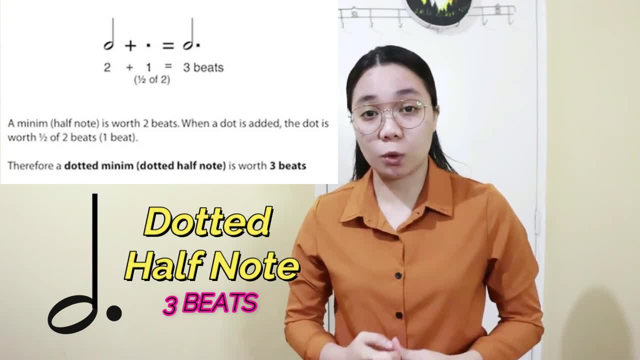 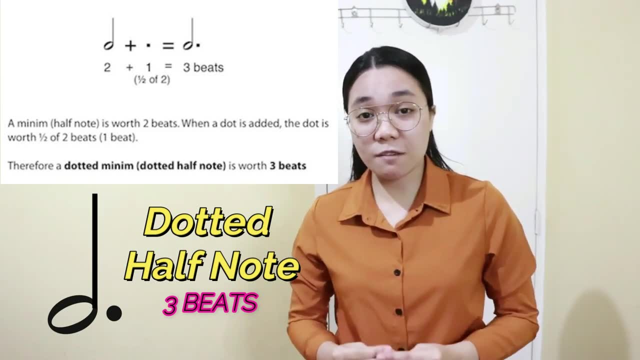 Because the value of dot is half of the value of the note being placed within. Let's say, for the example of half note, We all know that the time value of half note has 2 beats And the half of 2 is 1.. 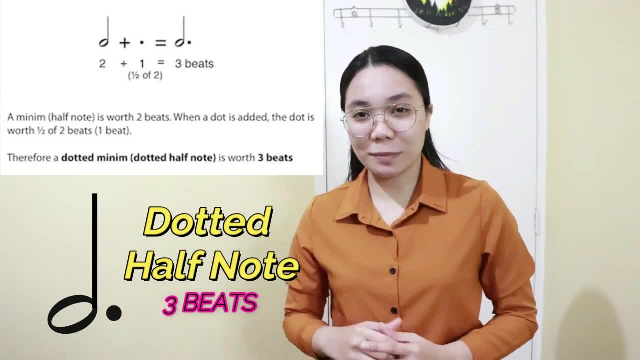 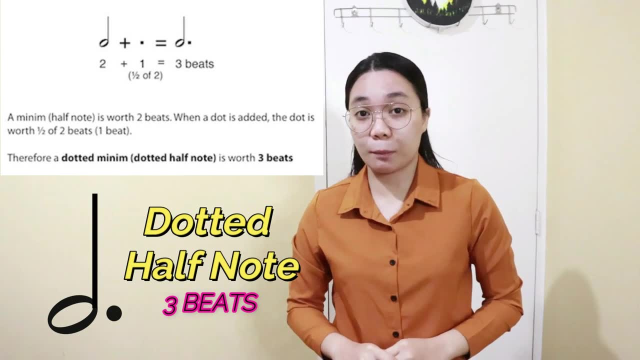 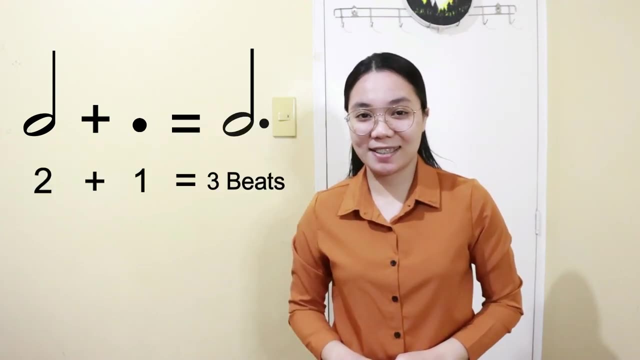 Right, Okay. Therefore, For the example of half note, we will put the value of dot. Just remember, the dot is half of the value of the note or rest being paired. So if we see a dotted half note, it receives 3 beats. 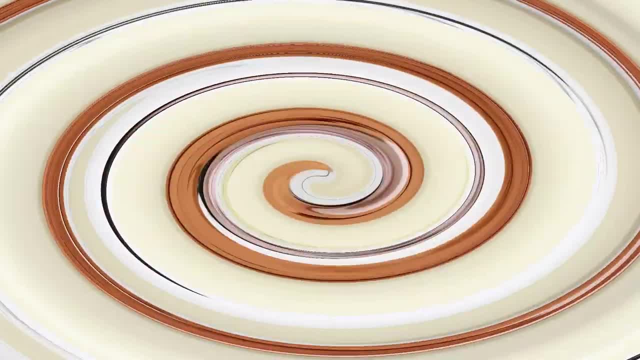 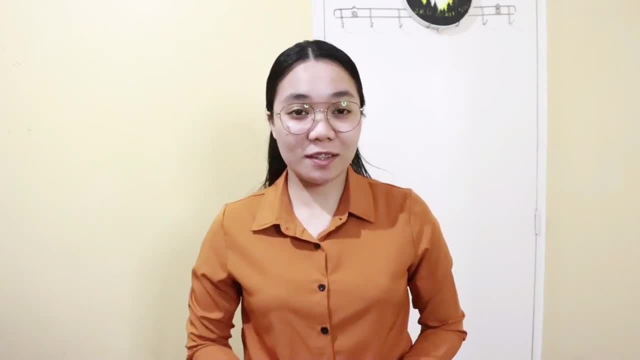 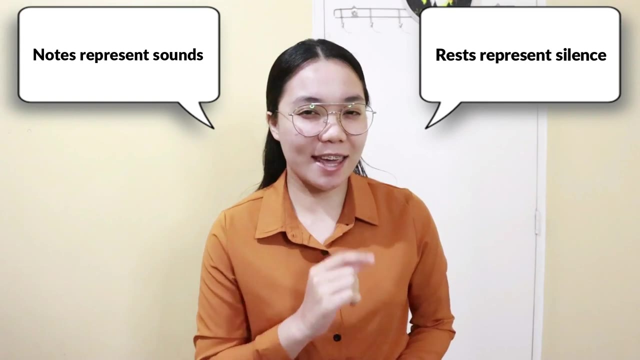 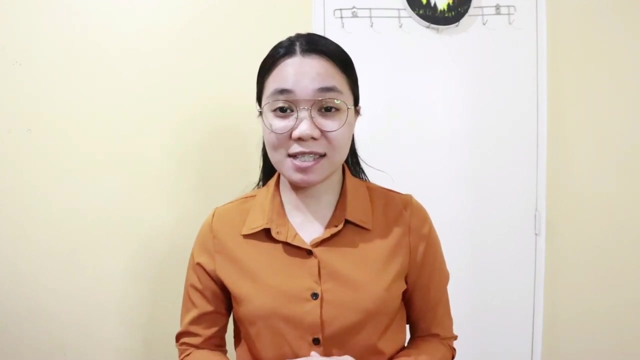 So look at this example. Now let's have the summary or recap of what we discussed for today's lesson. Just remember that notes are the representation of sounds, While rests are the representation of silence, And we should always remember, when a dot is placed beside a note or rest, its time value. 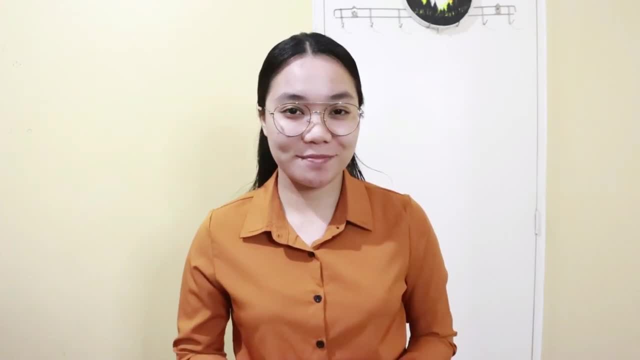 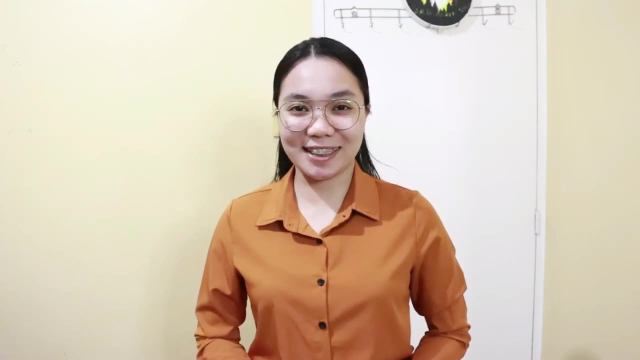 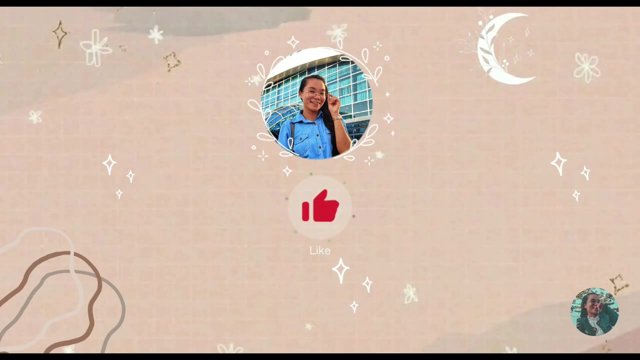 increases by half of the original time value. And that's all for today. If you have learned something, please subscribe to my channel. Thank you for watching. See you in the next video.